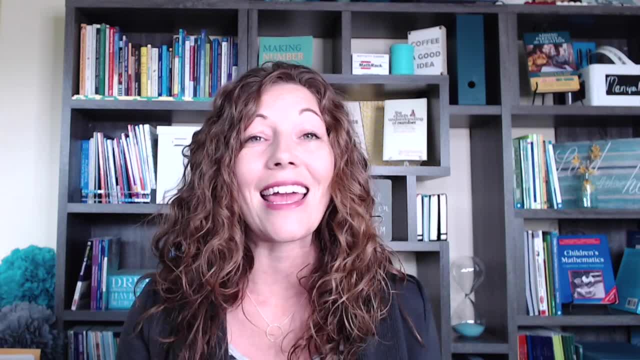 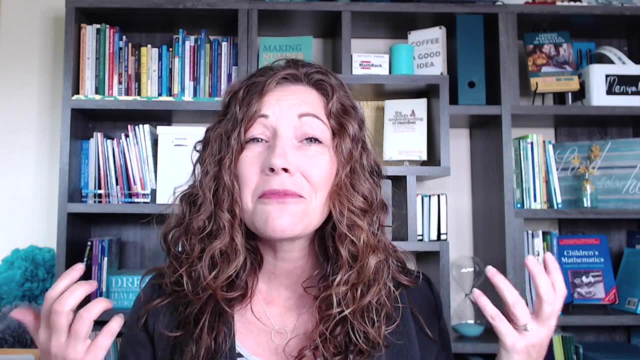 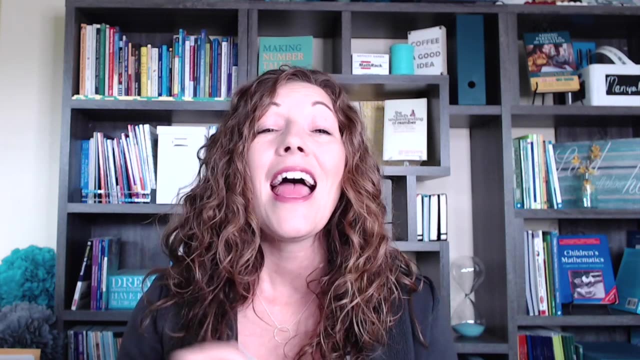 oh my gosh, that was amazing. So last week I encouraged all of you to kind of to ditch that textbook. But when you do that, what's next? I'm Kristina Toneval, the Recovering Traditionalist, and I hope you stick around as we delve into how to teach elementary math. 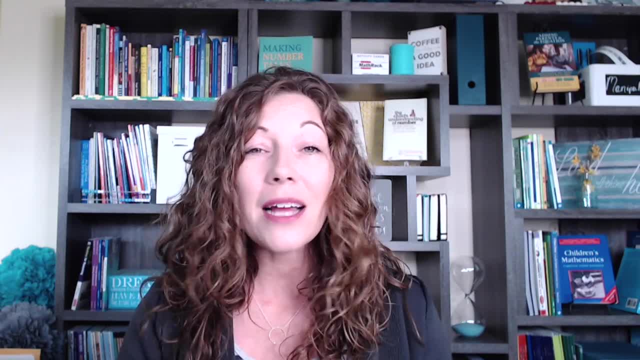 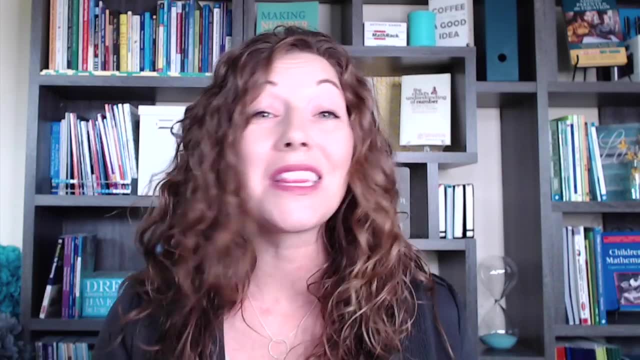 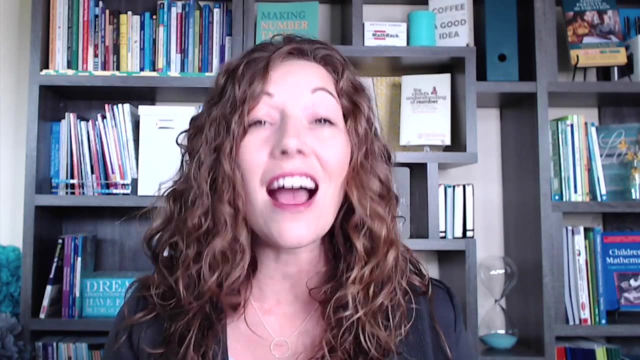 without a textbook in our quest to build our math minds, so we can build the math minds of the students. Now I've got to say I don't like making recommendations just based off my opinion. I like to back it with research and there's lots of research articles and books. 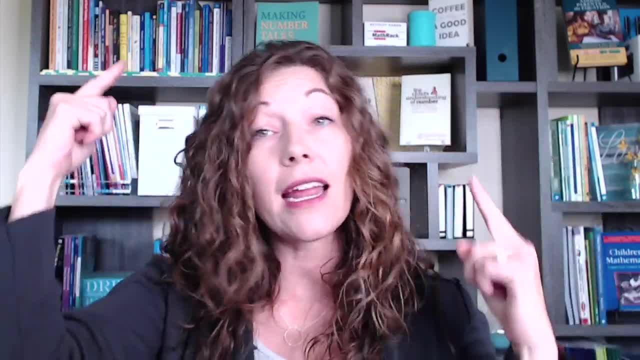 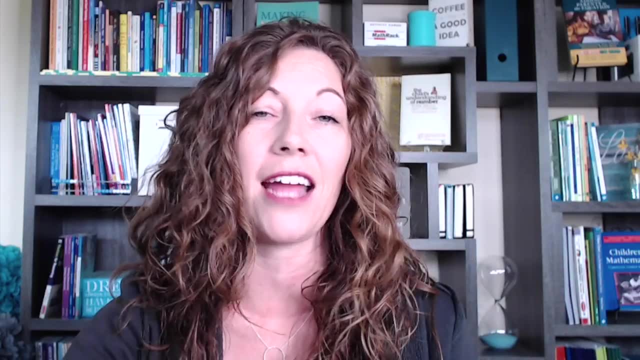 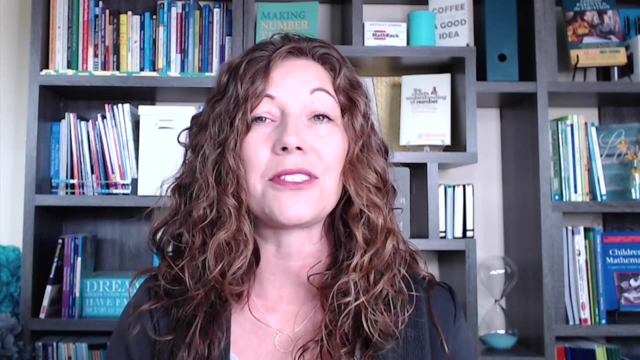 that I could point you to. Like, if I point anywhere, it would be awesome, right, But I had really hoped to kind of point you to one place to find the research. I went to my go-to place, which is the IES What Works Clearinghouse, hoping to find one of their practice guides that outlines 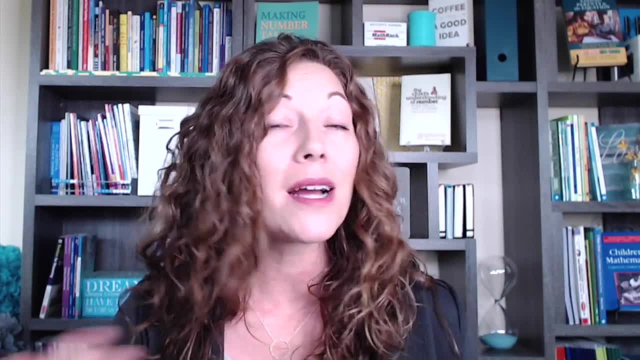 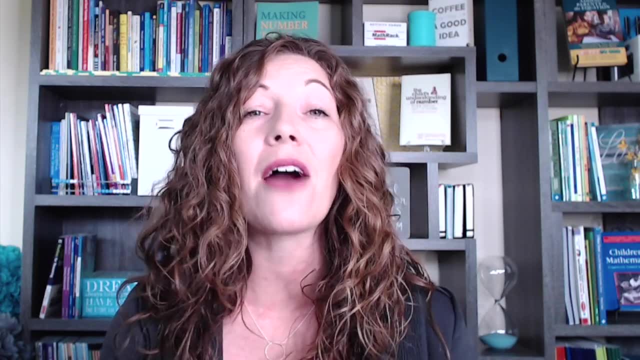 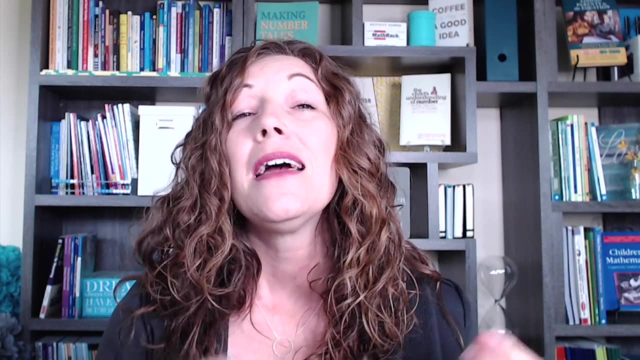 what works for elementary math, But there wasn't one. I will link up what they do have and one of my favorites, which is all about what works for students who are struggling and in need of intervention in elementary and middle school. But what I tended to learn from that was that the recommendations they make in 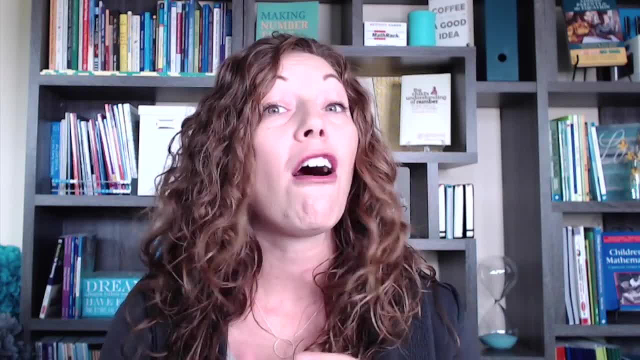 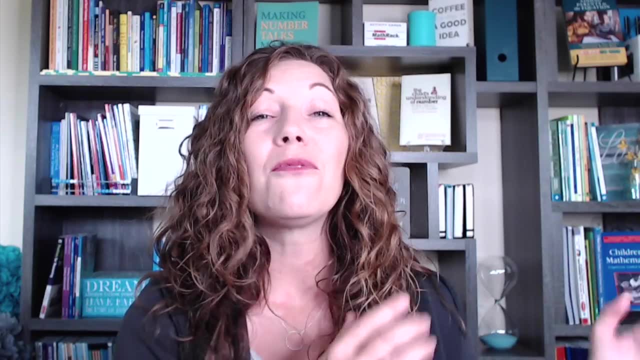 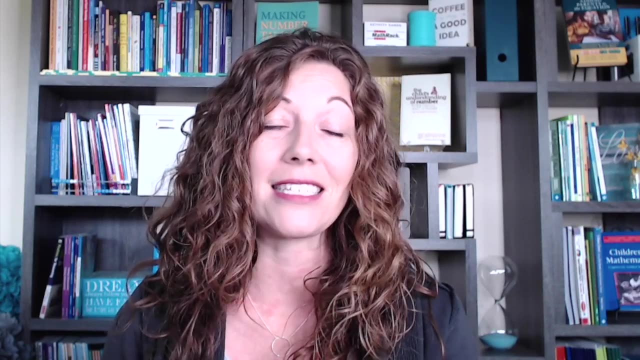 that document really are things that work for all of our students, not just kids who are struggling. So some of my recommendations today come from the books behind me, but some also come from the IES What Works Clearinghouse Practice Guide Assisting Students Struggling with Mathematics, which I will link to all of that right. 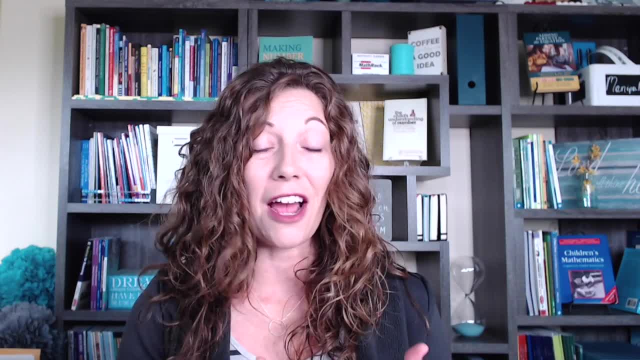 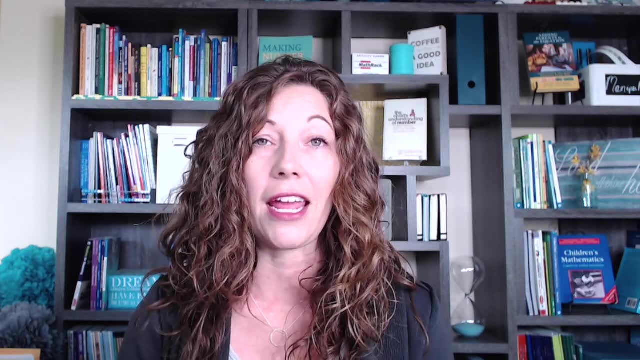 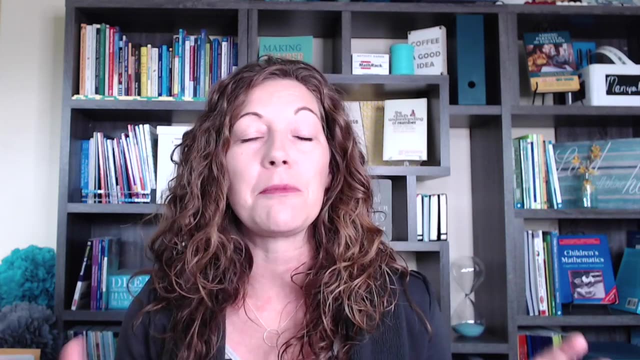 below this video. Now, the first thing that I want to start off with is: it is so important that you understand the progression of student learning Now. we are often told that the standards are our guide. textbook people will always tell me: yeah, the textbook isn't our guide, Our standards are our. 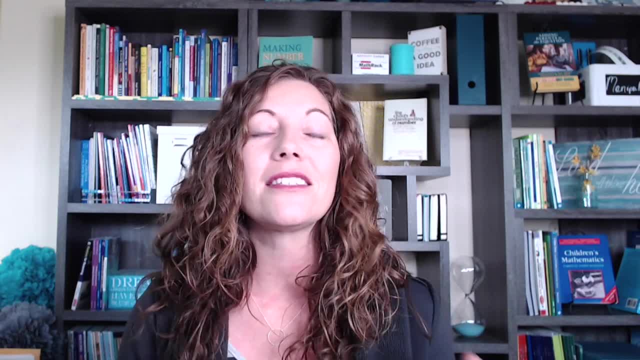 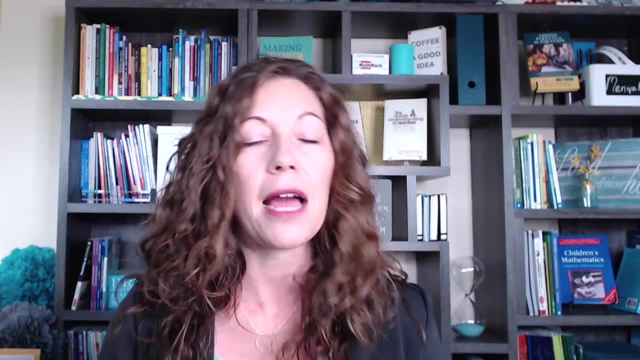 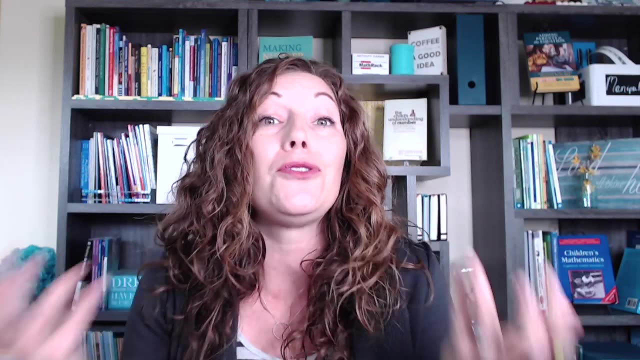 guide. But I like to push back even on that, because our standards only really tell us the end result. It'll say things like multiply two digit by a two digit number. It doesn't really tell us all the stuff that kids have to understand in order to be able to do that thing. So what the 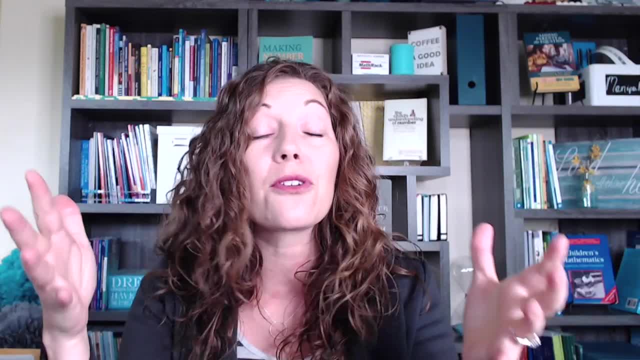 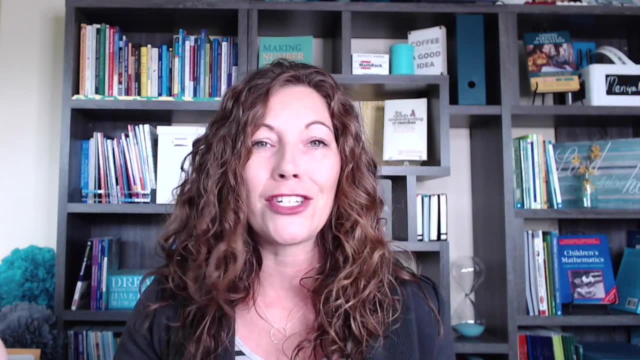 progressions are is they tell us how kids progress to get to that understanding. Now, they are messy. They are not normally a progression, And so there are a lot of people who don't call them progressions. So I like to call it a progression, but you'll hear other. 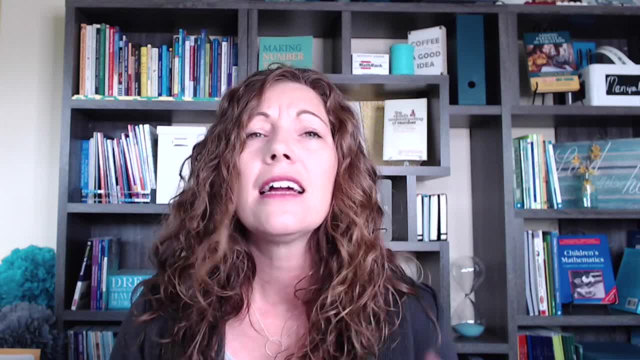 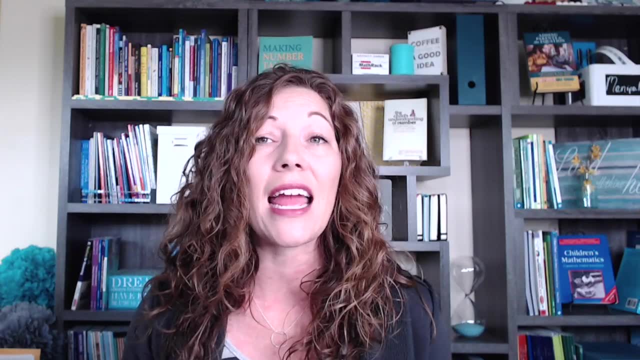 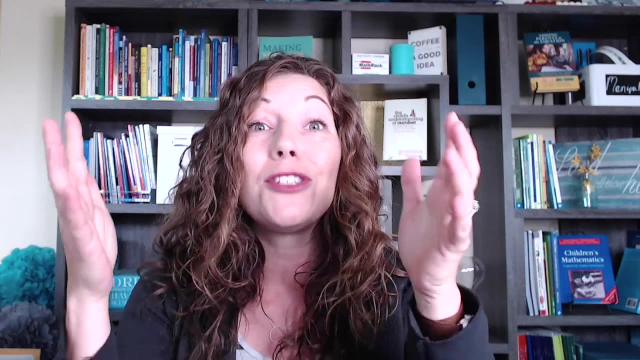 people like Kathy Fasno, who calls it a landscape for learning, Clements and Sarama call it a trajectory. I don't care what you call it, but you do need to understand where your students are, where we need to get them and how do we help them progress to that end point from where they 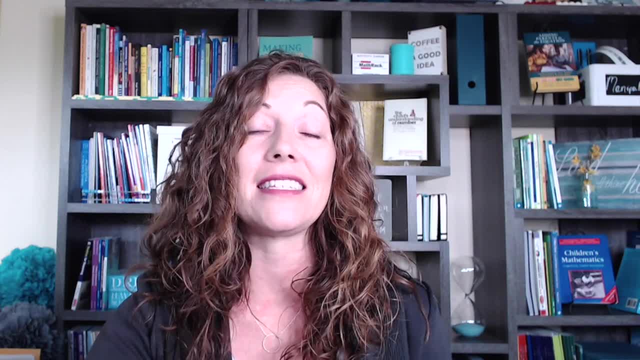 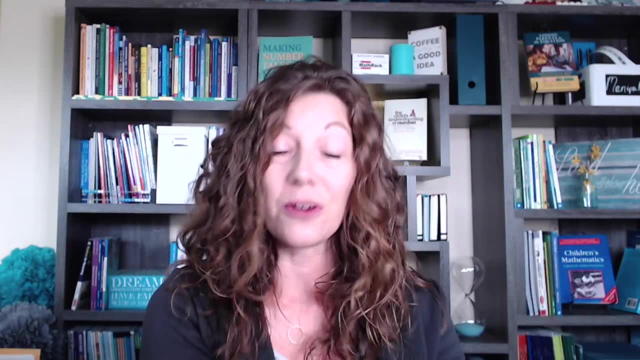 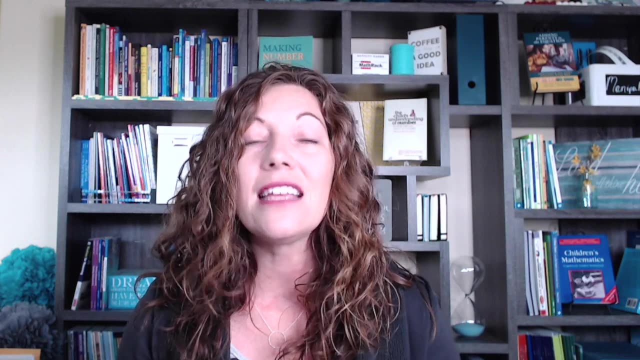 are. So I have three big things that if I could design a curriculum- which I don't want to because it's all dependent upon your students- but if I could design a curriculum, it would be around these three things, And these three things are things that if we include these three things, 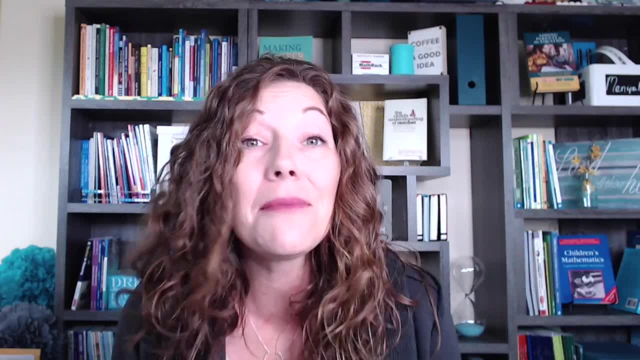 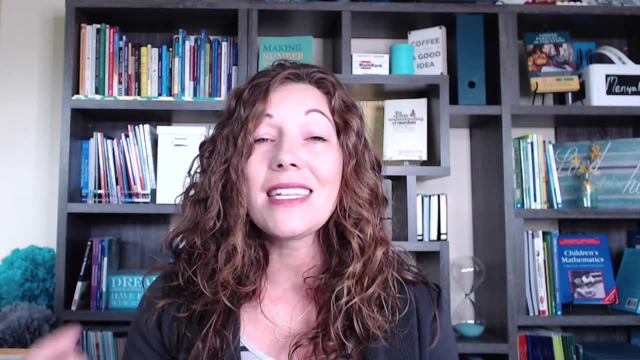 I don't really feel like we need to include anything else. I don't know. Let me know in the comments. Let me know what you think about this. So my first one that you need to be doing into the classroom is having a focus on number sense. 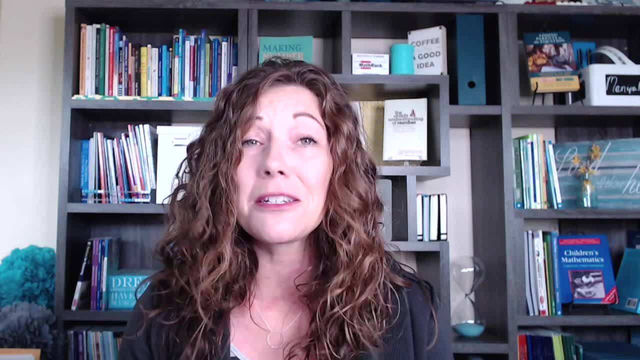 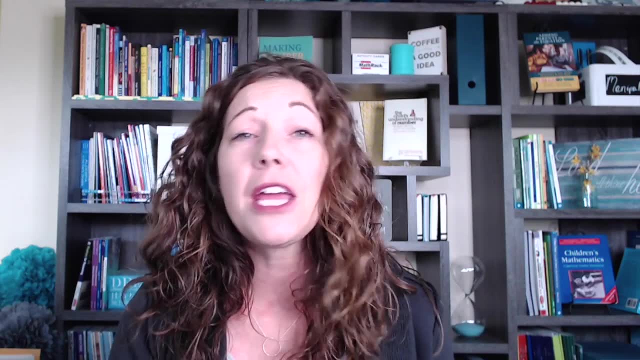 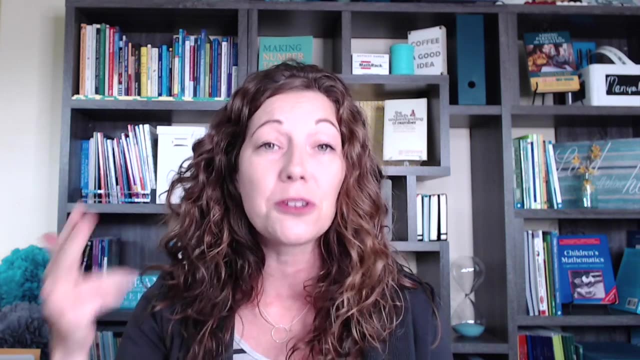 not number skills. Okay, Let's be a little bit clear on that because, let's be honest here, The focus in elementary school is on the concept of number. We aren't spending months helping kids learn and identify their shapes. We are helping them add, subtract, multiply. 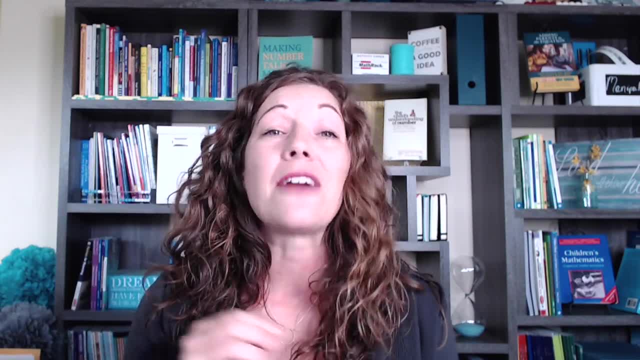 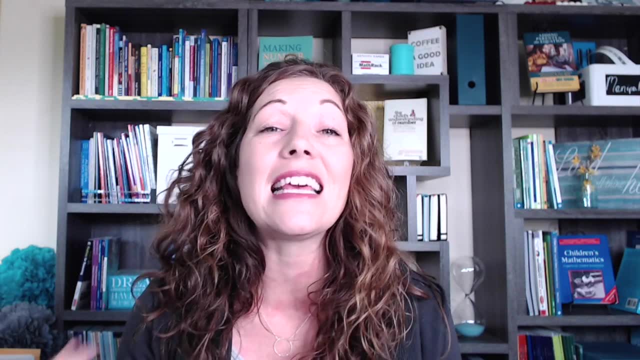 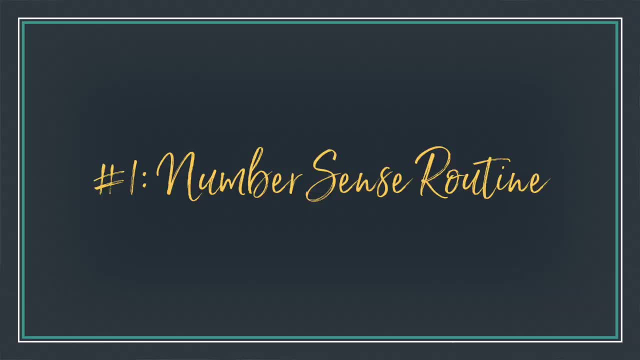 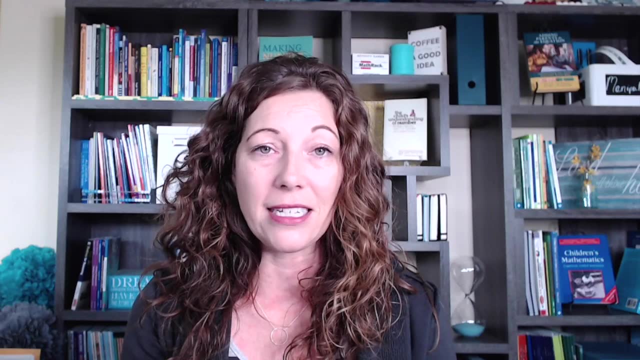 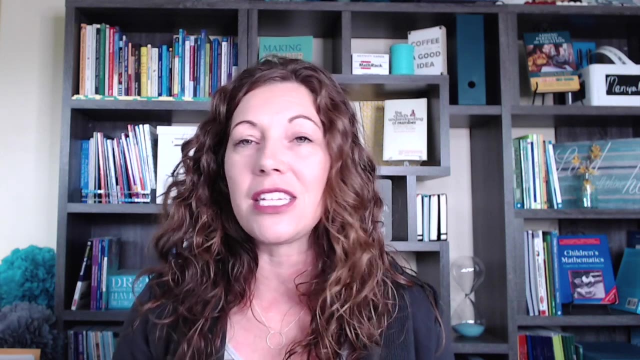 difference. So my first recommendation on what you need to be incorporating is building some sort of number sense routine into your daily practice. So I'm going to switch over into a different screen and we're going to talk about one of my favorite number sense routines. This is: 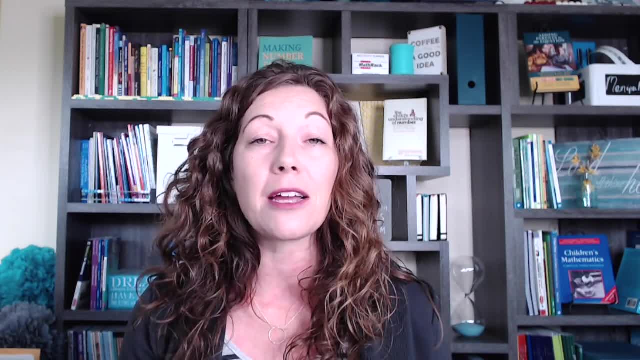 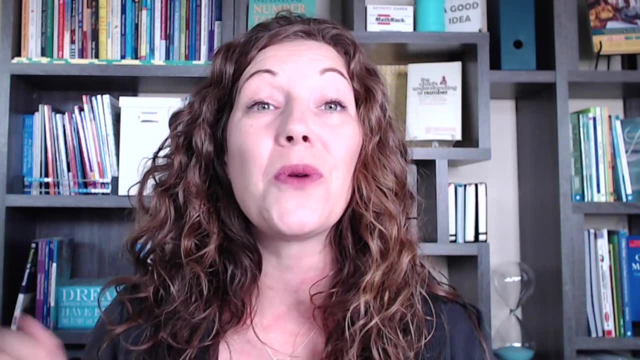 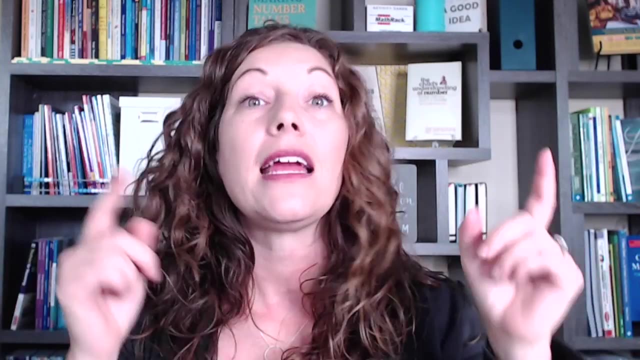 not the only thing you should do. There are lots of other recommendations, which reminds me to tell you that you need to grab the download that is linked below this video. I am putting together my guide for you. It's not my guide, It is your guide on how to teach elementary math without a textbook. So these recommendations that I'm going to talk about are going to be in the description of this video. So I'm going to talk about how to teach elementary math without a textbook. So these recommendations that I'm going to talk about are going to be in the description of this video. 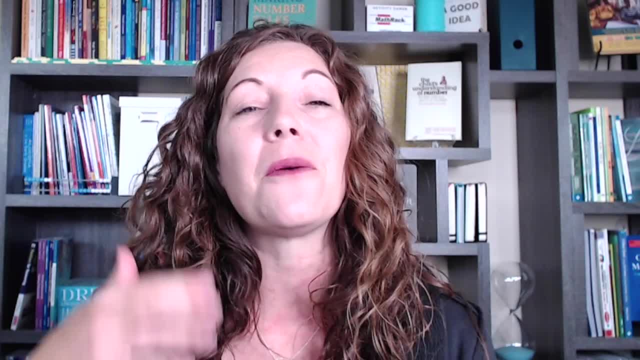 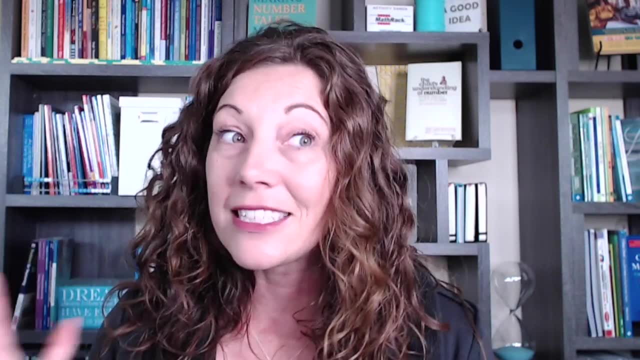 giving you are in there, along with some extra info that we're going to be talking about over this whole series that I'm doing about teaching elementary math without a textbook. It's all going to be added into this whole guide that you're doing. There's going to be some spots for you. 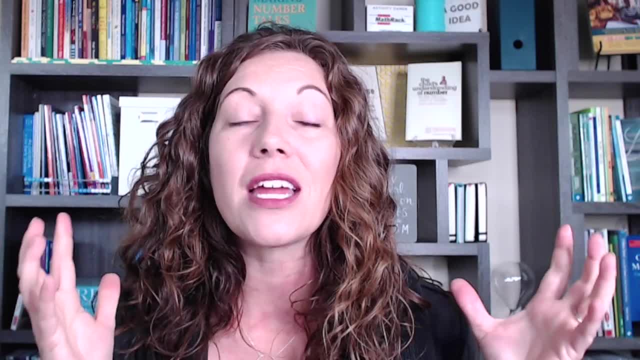 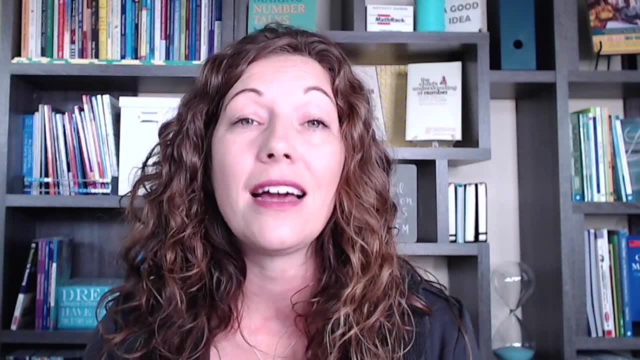 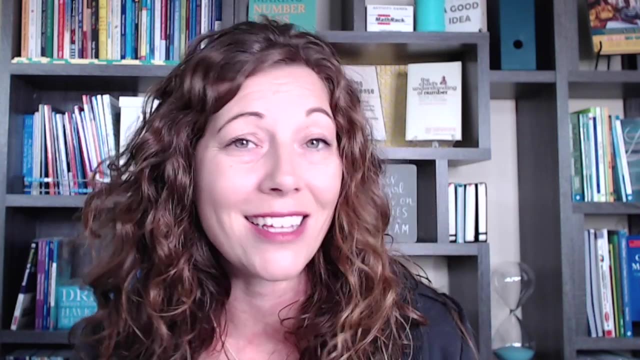 to fill in, Grab your download so that you can have your own guide on how you plan to teach mathematics without a textbook. Now you may do all of this, You may do some of this, but I hope you don't do none of this, because these three things are just so darn important And I 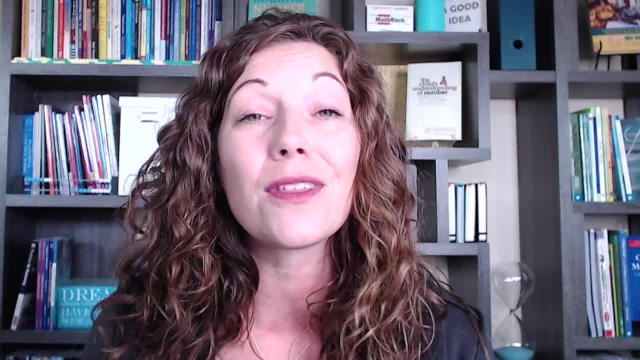 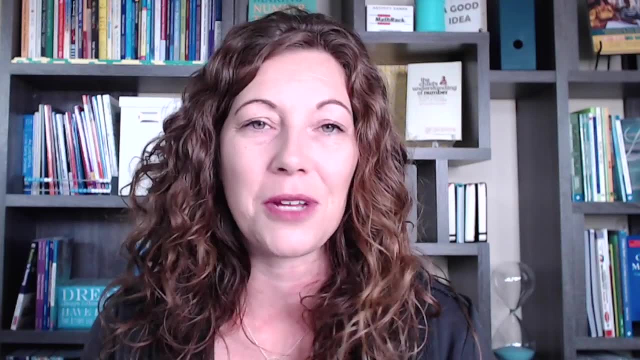 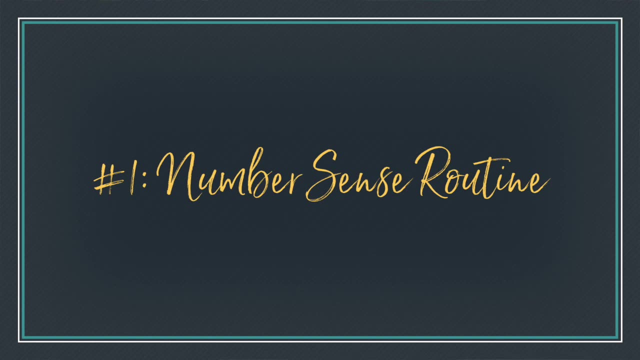 hope, throughout this video and the next ones to come through this whole series, I convince you of that, that we've got to stop focusing on a textbook and start doing these three things. Okay, so let's take a look at one of my favorite number sense routines. Okay, this is not a reminder, This is 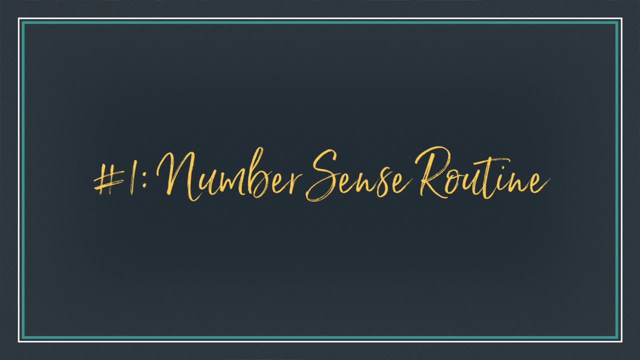 not the only one. I will reference more inside of that guidebook that I am going to be talking about. I am asking you to download. So first thing I want you to take a look at is think of number sense routines that you might already be doing. It does not have to be this number sense routine that I 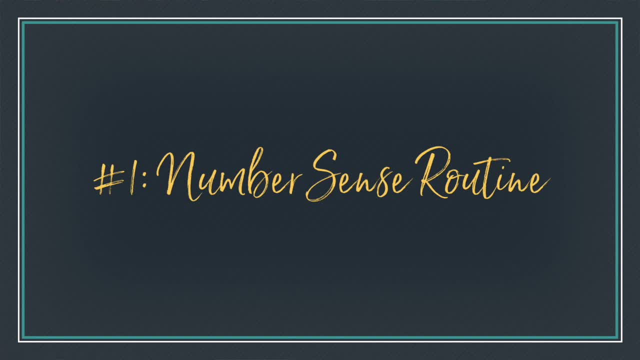 am going to suggest. So our first one that I want to recommend to you is my favorite number sense routine, which is a number talk, or you could do a number string Now really quick, down and dirty. Here's the deal. Here's the difference. A number talk is when you give kids one problem, one visual, whatever it. 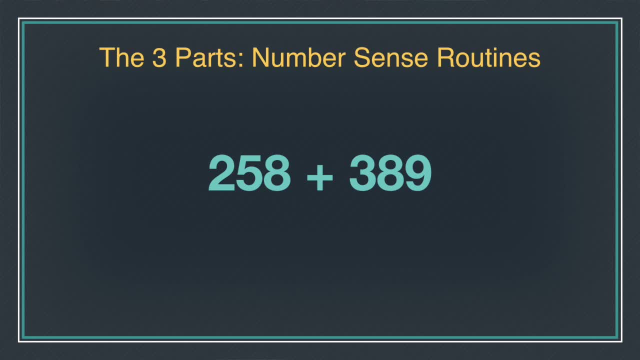 might be and you ask them to solve it in any way that they can. Okay, that's the piece that I want you to be doing. there is that they solve it any way they can, And then you have them share the different ways that they solved it and then talk and discuss about those different ways, Compare, 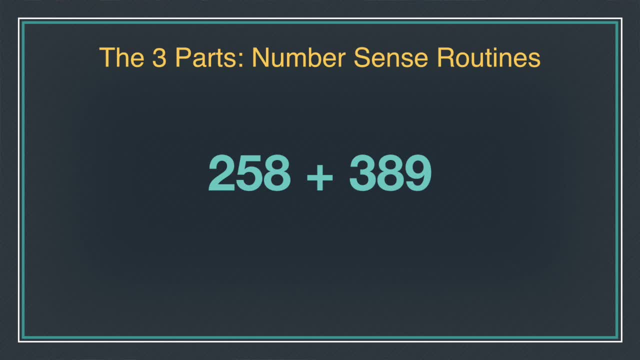 contrast. what was the same, what's different, all that fun stuff. However, if you've ever tried a number talk and the kids kind of all have the same way of doing it, then a number talk isn't the best thing. Instead, what I might suggest is a number string. A number string starts out with a. 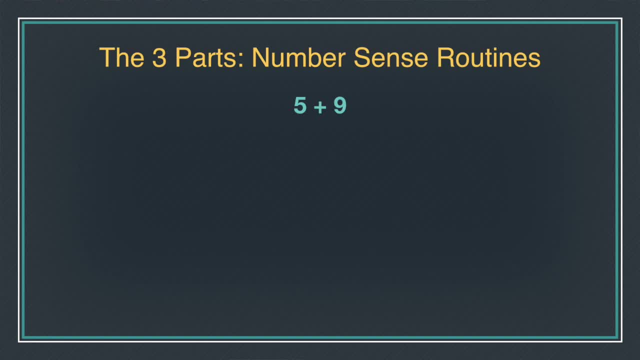 simpler problem that most of your kids might know, or maybe it's a problem that some of your kids are still working on, like this: five plus nine, And then it's a whole string of problems that you show one at a time and you're 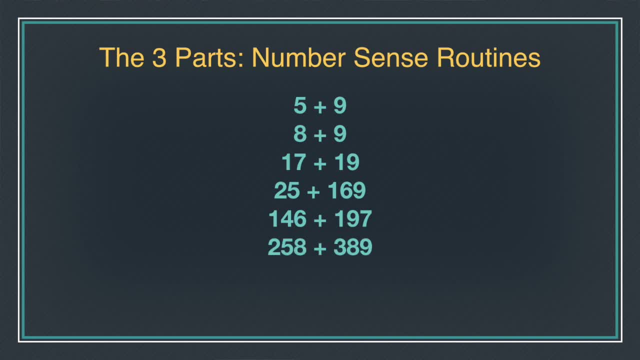 leading them into this final problem. Do you see where? this final problem is the exact same one as the original one that I did on our number talk, But instead of just putting up the one problem there now, I've led them, using this string of related problems, to come up with maybe a different. 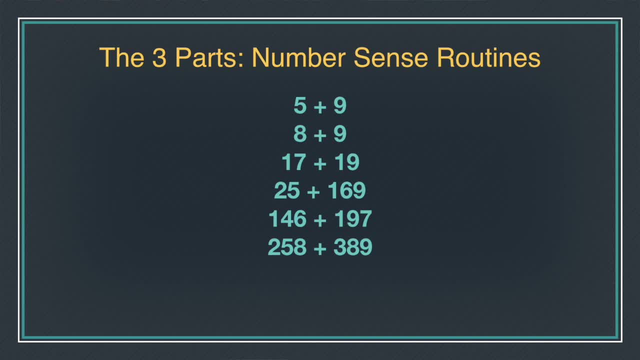 strategy that students had not ever had before. So number strings is a series of problems and you're trying to build a relationship or a strategy. Number talks are great if your students already have strategies built. they see relationships and you're just having them. 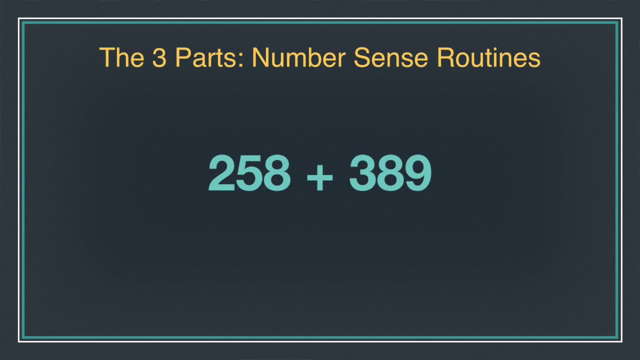 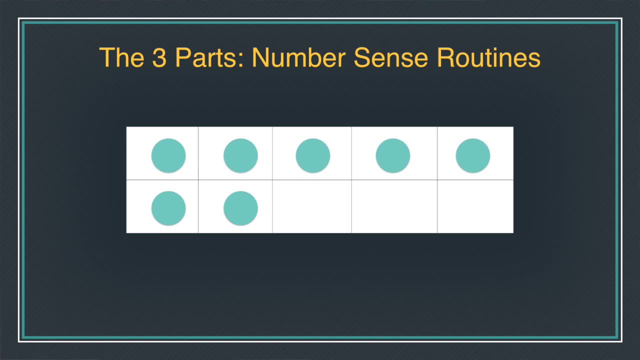 talk about the different ways they're seeing it. So a reminder: it does not have to be just problems like bear problems, it can also be visuals. However, if you're doing a visual and you're doing a number talk, this is not a great visual to do a number talk, because 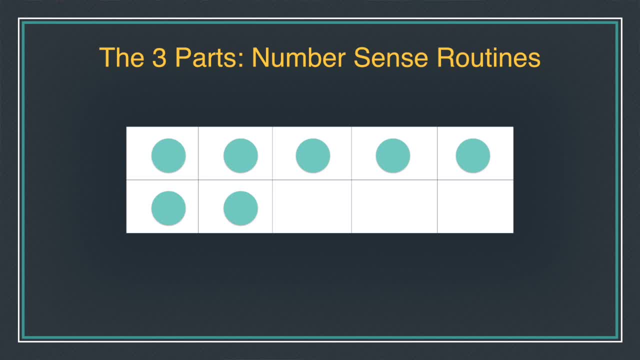 kids need to have something to talk about. There's not a whole lot to talk about here. It's a five and a two. Some kids might see a four and a three. There's just not a lot of variance that kids will see. But if I take those same dots and put it into this random 10 frame like this, there is so. 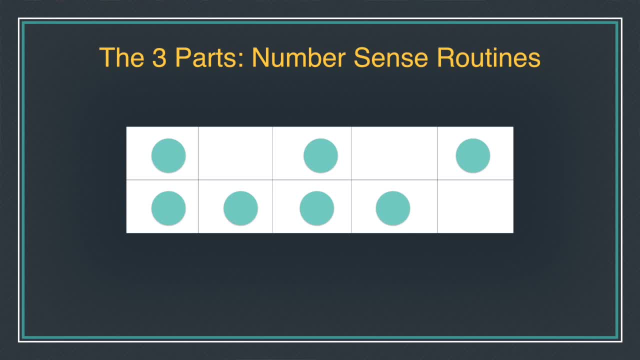 much more discussion that happens here, because kids will see it in so many different ways. So when you're doing a number talk, it needs to be something that will bring up different ideas, different relationships, different things that kids are seeing, and then you have a discussion. 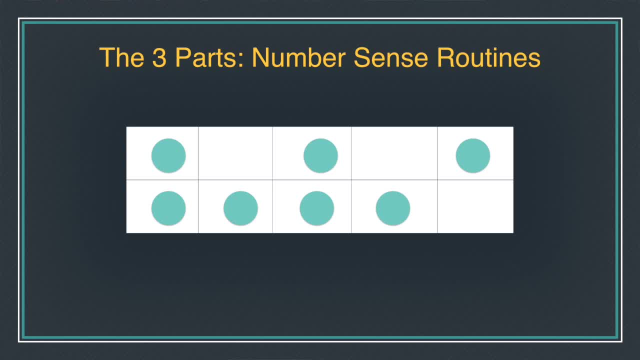 about that. It doesn't matter if it's a visual or a bear problem. Okay, that's an idea of a number talk. So number talk, number strings. those are some of my favorites, But again, in the download I'll reference more and we will be doing future videos coming up about more ways to incorporate. 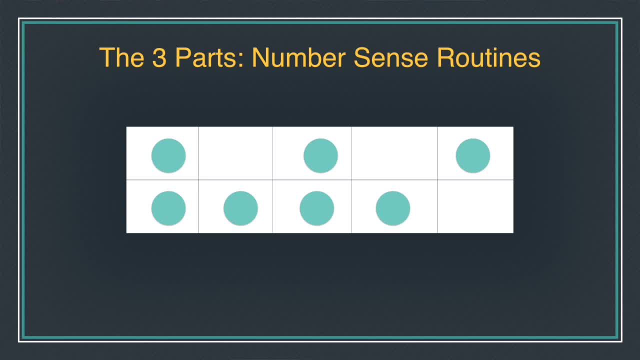 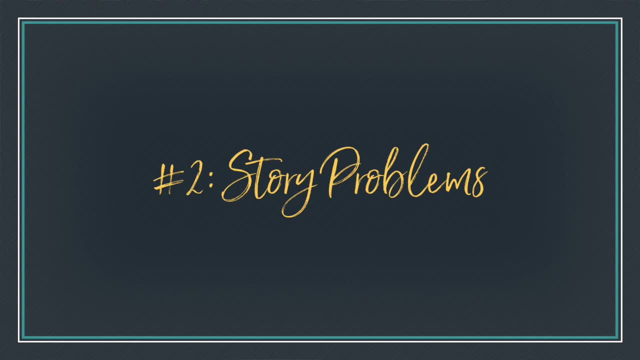 number sense and do number sense routines in your classroom. So our next idea that I really want you to consider incorporating into your classroom is number sense, And I really want you to consider that in your classroom is the use of story problems. There is not enough of this, And if your 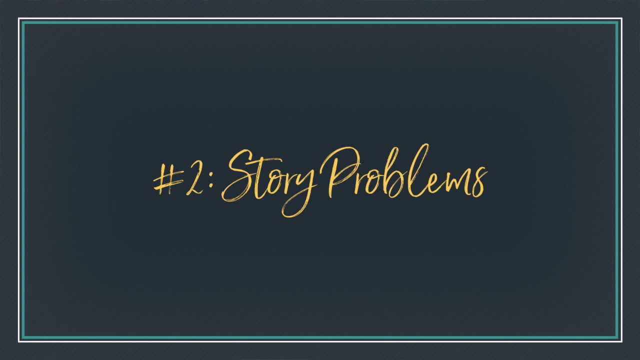 textbook does use story problems, it is often done in a very procedural way. It'll give this great story problem and then it'll tell the kids: step one, do this, step two, do this. step three, do this. That's not the best way to go about story problems. There's a lot of things that we will. 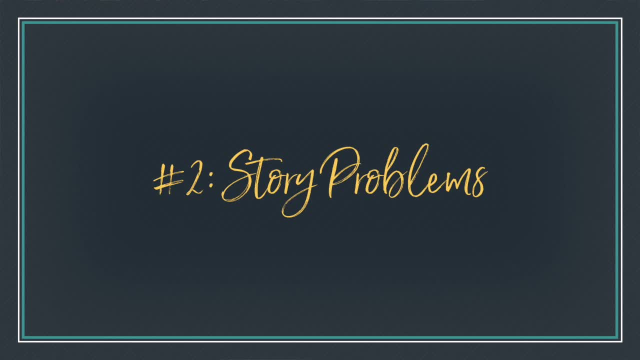 talk about in a future video- all about the research of cognitively guided instruction and how kids can use story problems in their classroom. So I want you to consider incorporating story problems in your classroom and how kids have their own intuitive way of solving problems. 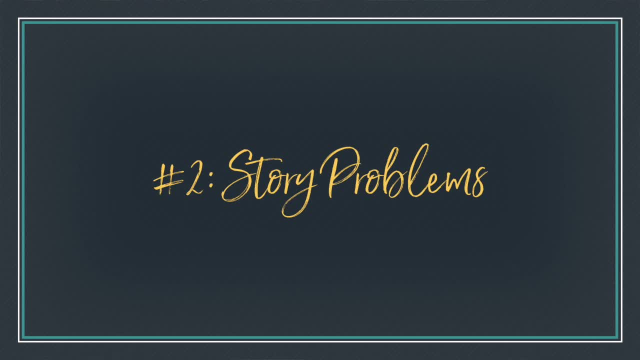 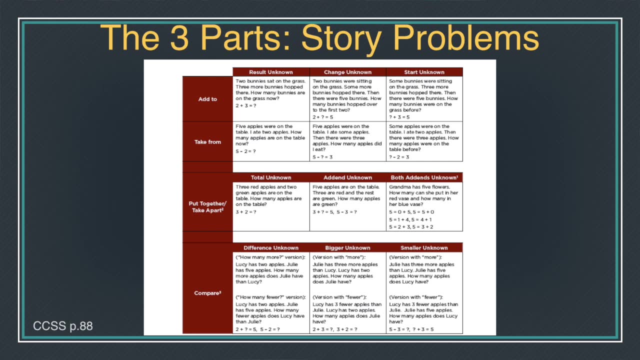 For this part of the video. I want to ensure that you all know about the problem type charts. If you are not familiar with these problem type charts, you got to go find them. Just Google: problem type charts. math problem type charts charts or CGI- cognitively guided instruction. story problem types. 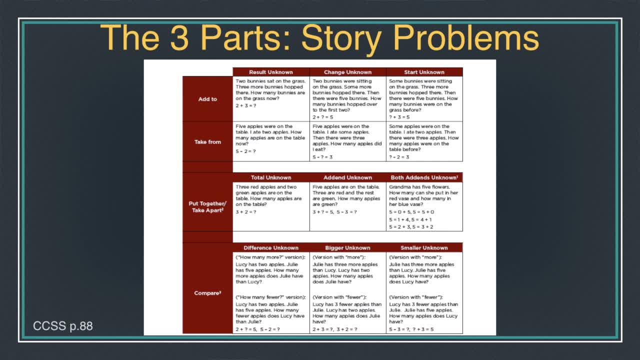 any of that. This is a screenshot taken from the Common Core Standards. This was in the appendix. I put the link in the description below. So if you're interested in learning more about story problem types, you can click on the link in the description below. I use this one because this: 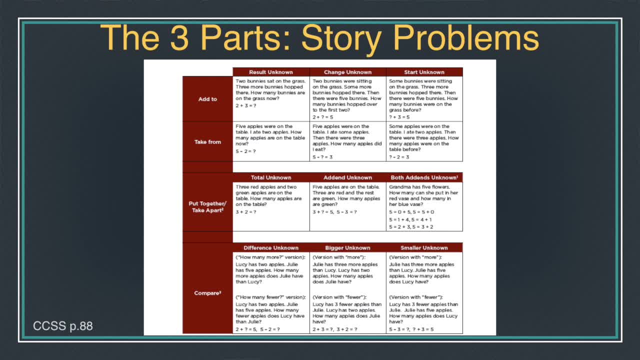 might be more familiar to everybody besides the cognitively guided instruction version, But this chart is not for your students. Let me repeat that This chart is not for your students. This is for you to know about the different story problem types, and there's a whole lot to learn. 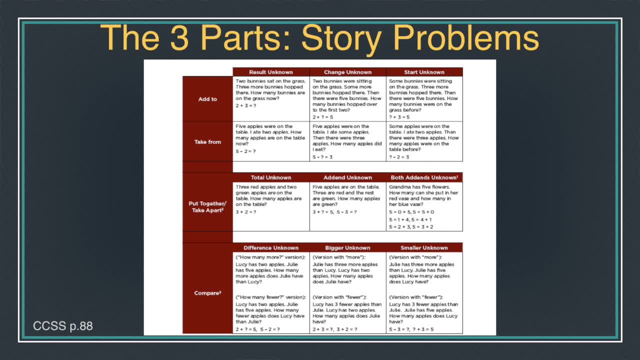 about why some of these are easier for kids to solve than others and why some of these are, even when you're using the exact same context and the exact same numbers, Some kids can solve some of these types and not others. It's a whole. it's a progression, right? We're talking about this. 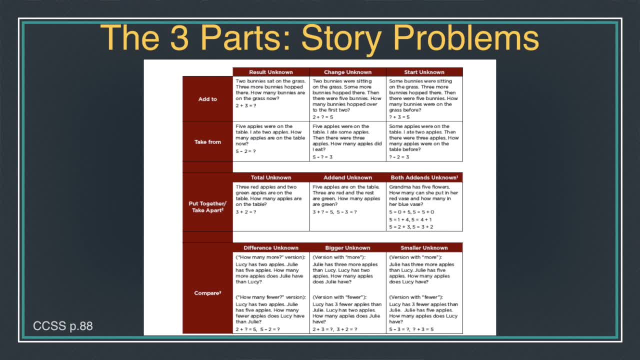 progression again. So kids will solve story problems using a type of progression. Some of these are easier, some are harder, and we need to have that knowledge about story problems so that we know: is it the story problem that's causing the issue, or is it the mathematics, the numbers? 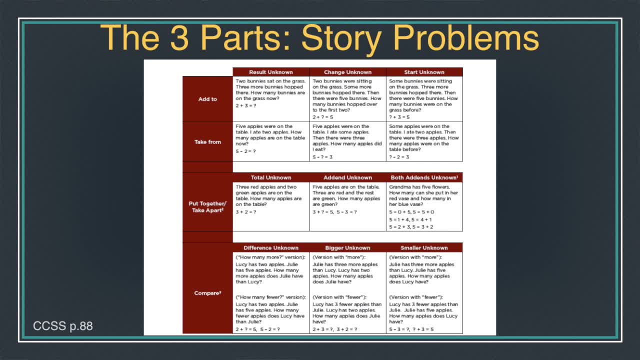 that are in there. So we need to have that knowledge about story problems so that we know: is it the that are in there? Because sometimes kids will be able to solve an add to with a result unknown problem with bigger numbers, and yet they can't solve this bunny problem where it's blank. plus. 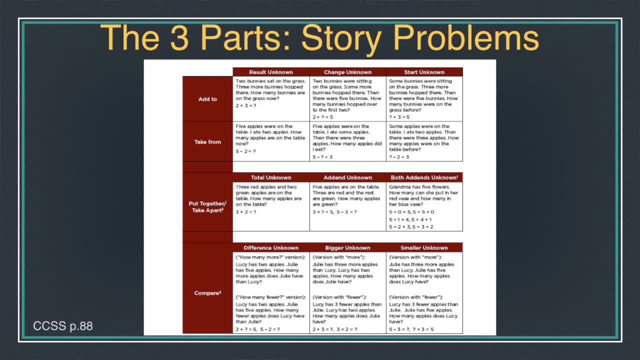 three equals five, right? It basically boils down to that. but they can't solve it because it starts out with some bunnies were on the grass and kids don't know how to start when it says some and they're asking you: how many is some right? Have you ever had that? I have lots of times. 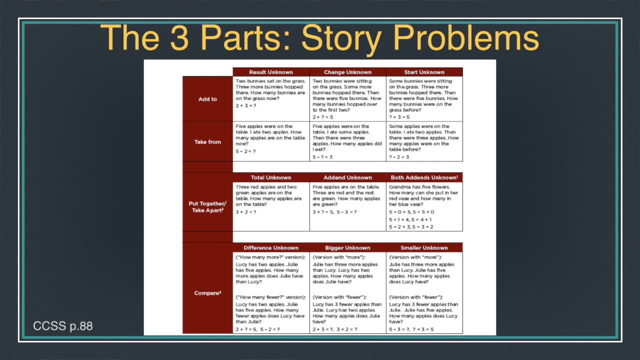 so that's why I'm going off on a rant about it, But the idea is that you need to understand these story problem types to ensure that your students are being exposed to these problem types, but also to understand that the problem type may be why a student is not able to solve it. It might not have 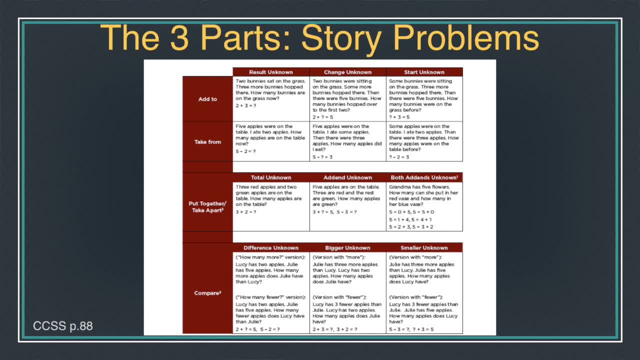 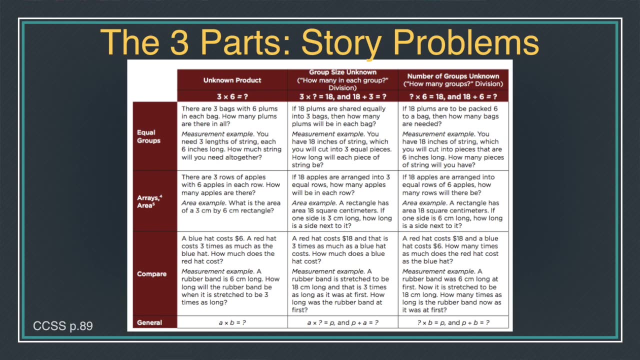 anything to do with the numbers, but just the way that we write the story problem can impact whether or not a kid can solve it. And yes, we do need to have kids be able to solve all of these problem types. for the multiplication and division problem types, Kids and when you're going into multiplication, 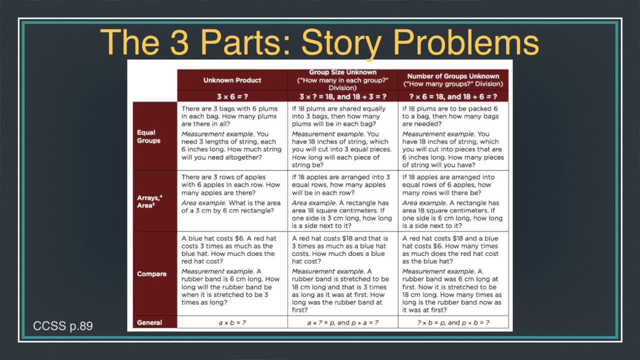 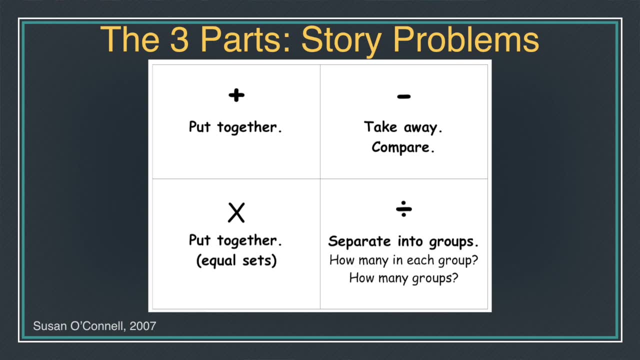 and division. kids need to be doing it through a story problem lens. They need to have the mathematics in a context, and story problems are a great way to make that happen. Now, I also love this little chart from Susan O'Connell that she kind of helps this get us away from the key words. 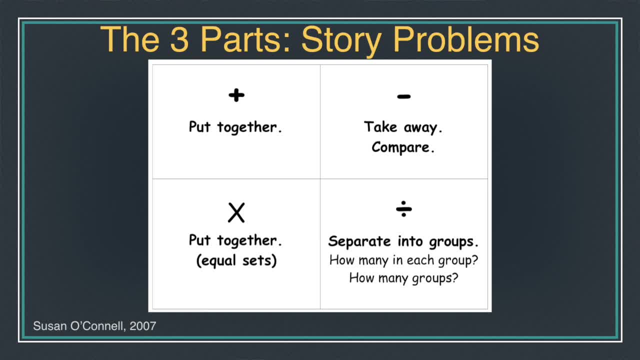 Key words is kind of the death of story problems. or story problems can be solved with key words, sometimes right, But if you really want to get into problem solving key words, don't do that. If you're having kids underline and highlight and circle, that is not problem solving, That's. 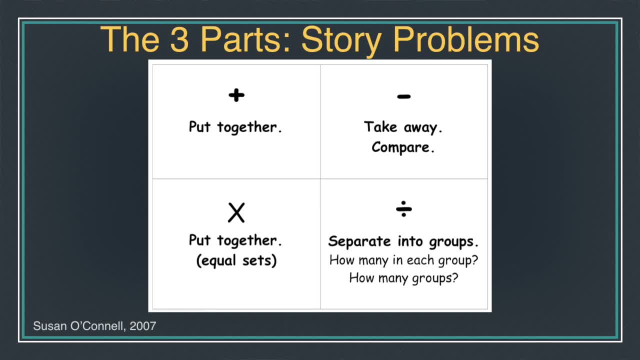 just pulling out information and trying to get answers. If you want to build true mathematicians, they need to be solving story problems in context, Using their own understanding, And one of the big pieces to help kids understand is this: key concepts, not key words. The key concept of addition is that you're putting things together. 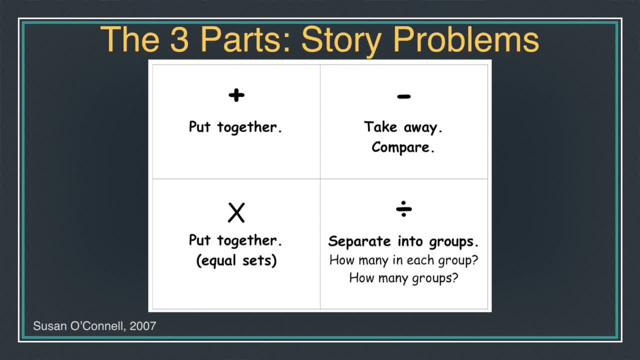 That's a key concept. It's not when it says all together okay. We'll talk more about all of this stuff in future trainings, but this is again just a brief overview of this information. All right, Our last one that I really want you to consider: 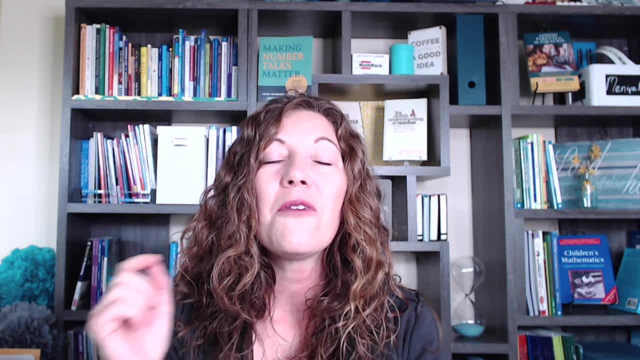 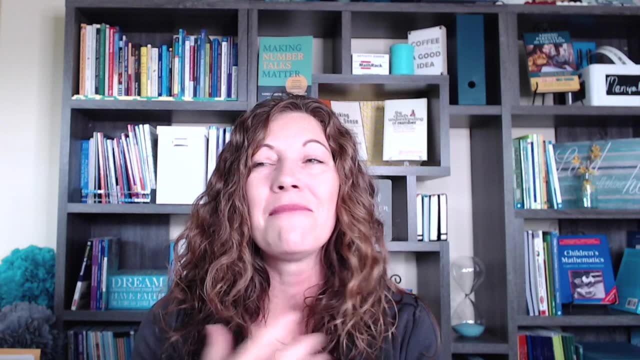 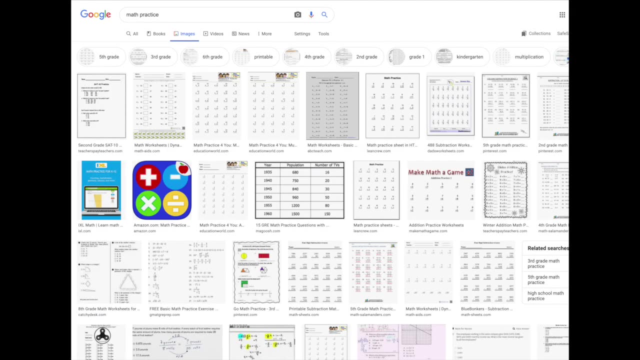 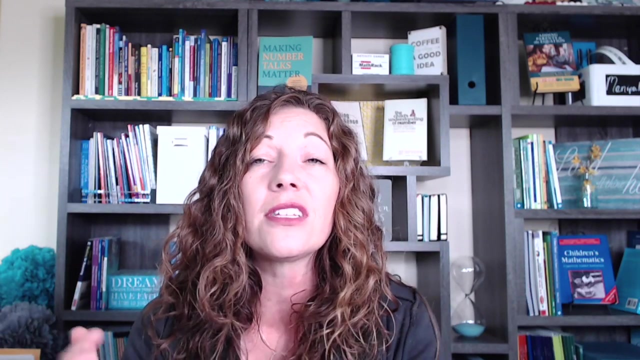 we're doing is practice. Now, practice is often kind of a bad word, I guess, in my eyes, in mathematics, because it conjures up this image, And even when you go Google it go Google math practice. here's what comes up is that it's worksheets, it's drill and kill, And so this. 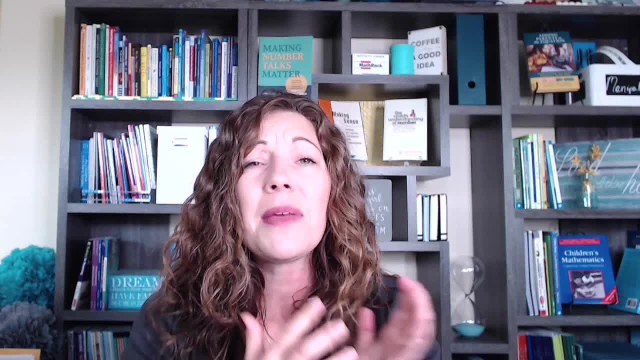 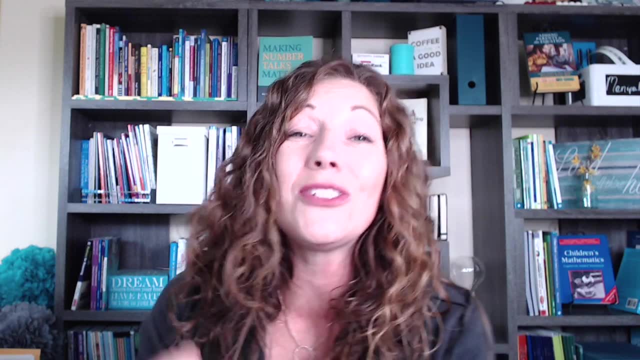 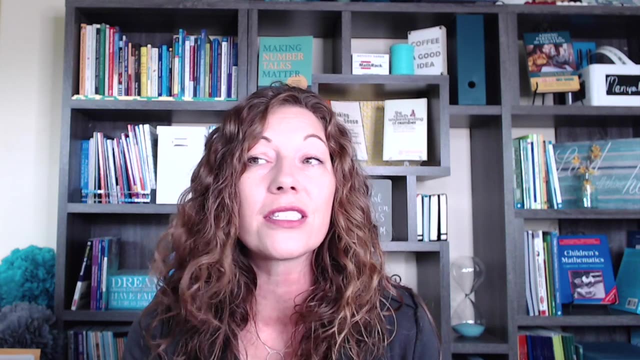 idea of practice we have kind of gone away from because we feel like it's not building that thinking skills. But man, kids still need to practice, right, That's how you hone your craft in. anything is that once you understand how it all works, you need to practice and get better. 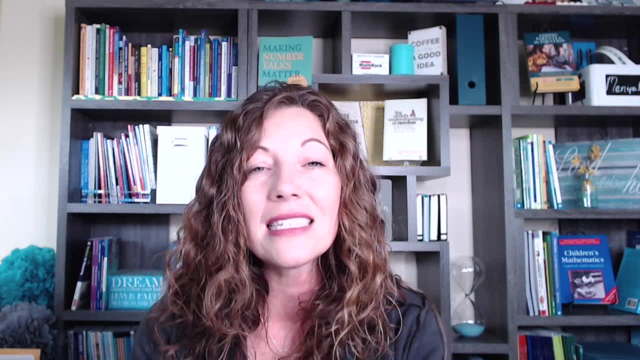 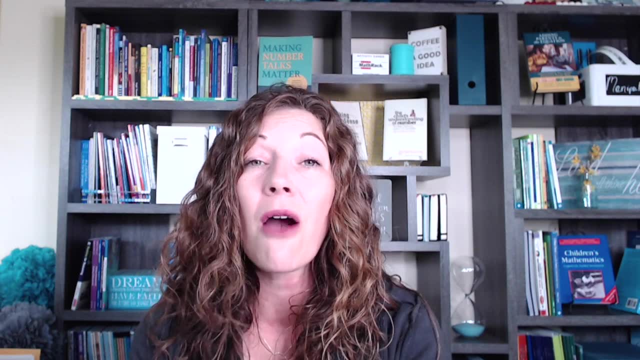 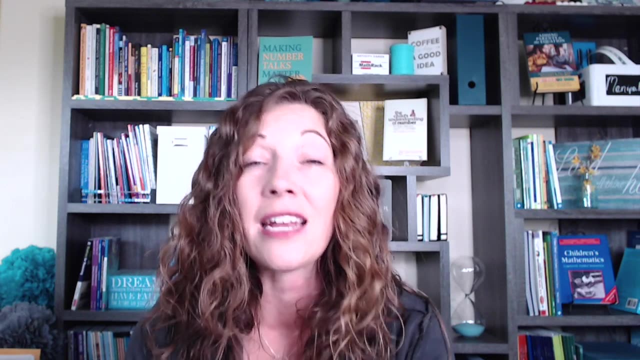 and more efficient at it. So practice needs to be a big part of what we're doing in mathematics, But I really want you to think about ways to make it fun. It does not need to be a worksheet. Math is not a worksheet and practice does not need to be a worksheet. So my third and final: 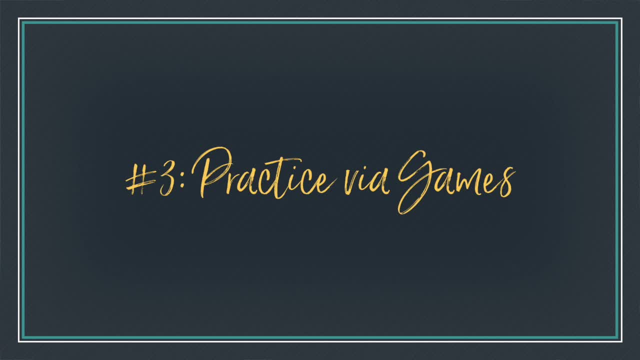 recommendation is to practice via games. Make it fun for kids. Now, I know that games can be scary, intimidating, a pain in the rear, however you want to say it, But games are such an important piece. Not only does it build mathematical thinking for kids, but it also builds mathematical thinking. 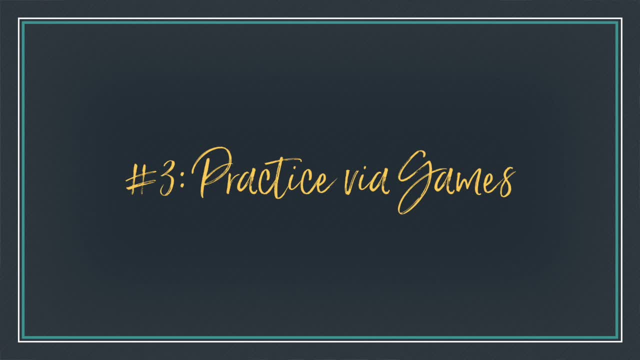 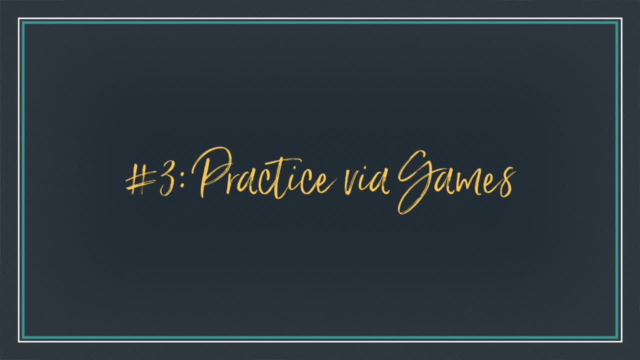 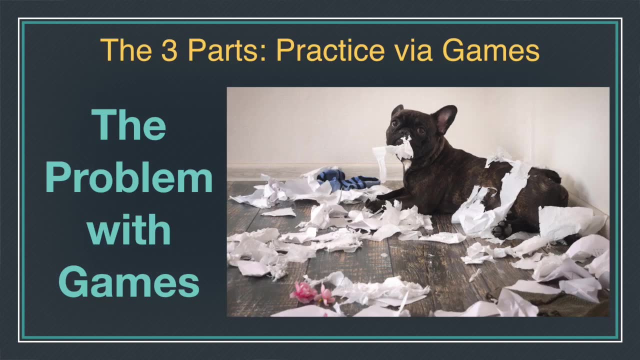 being played in home as much as they were in the past. So as much as you can bring in games, Now the problem with games is you have to teach them. Kids make a mess. There's stuff everywhere, So I want to encourage you to think about what I call evergreen games. Are there games that you 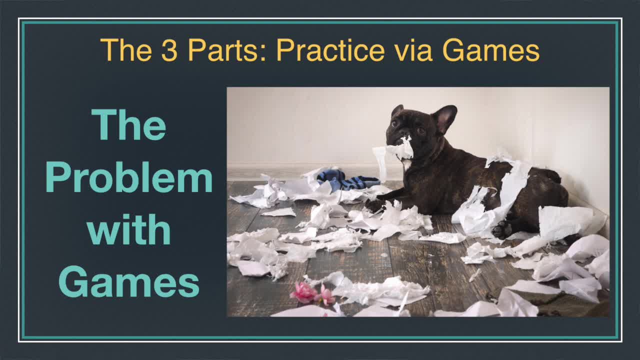 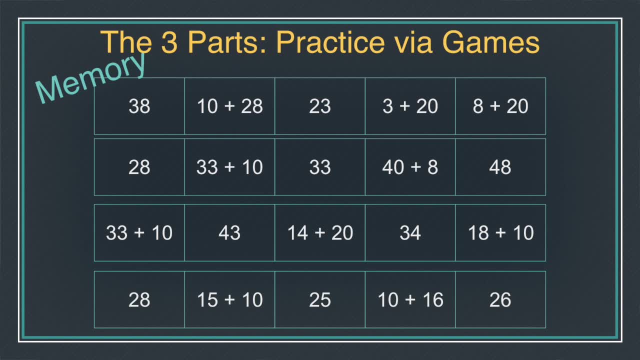 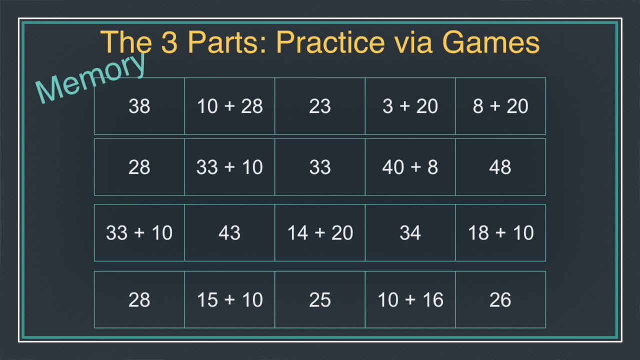 match, you get to keep those cards. But once they learn how to play memory, all you need are different decks of cards that are paired in different ways. So here's ones where you can make that have like an equation, basically 10 plus 28,, and they are trying to figure out the answer to. 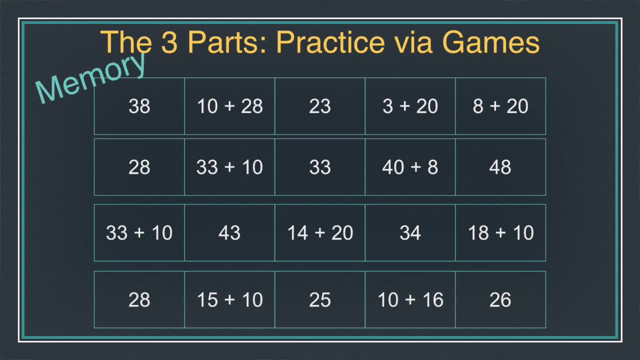 that. So the match is the answer to that. And then you have to figure out how to play memory And you can have visual ones, like just think of ways that you can create memory games and just switch out the content. Then it's a lot easier because you don't have to teach how to play the game over. 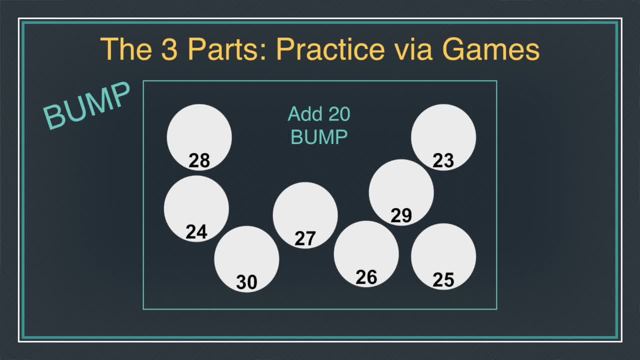 and over again. Another popular one is bump Bump's- a popular one that's been around a while. This is one where you roll the dice and then you add 20, and then you can put your game piece on that spot, Or I like to put these in little folders. 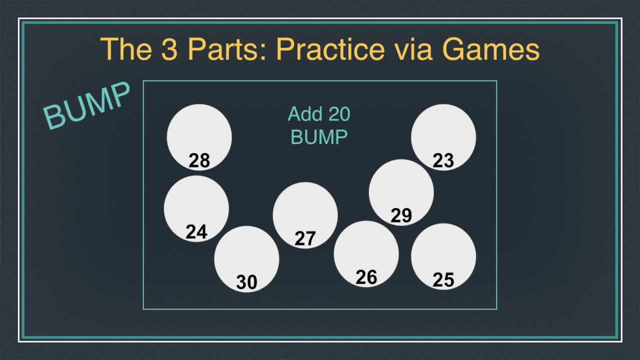 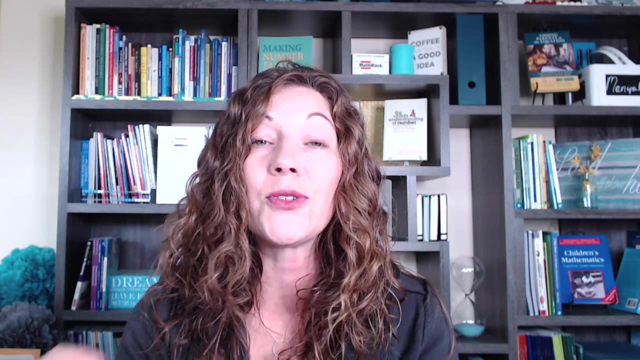 And then kids can use whiteboard markers and mark on them And if you get two marks on your spot nobody can bump you off. But if you only have one marker and somebody rolls that same amount, they can bump you off. That's the fun part of bump. So games are a great way to incorporate. 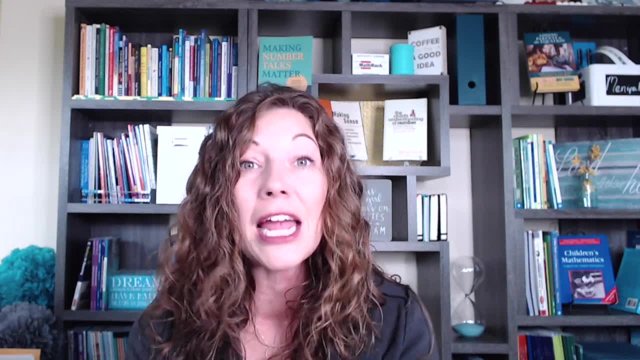 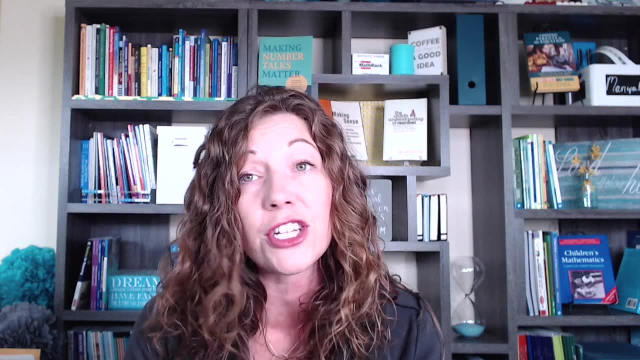 practice. Kids are getting tons of practice without even knowing that they are practicing. It is a fun way to build this mathematical practice to help kids become more efficient. The hard part, which is the hard part, is that you don't have to be so good at it. You don't have to. 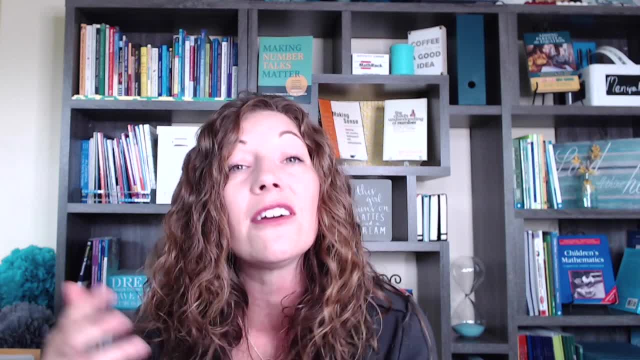 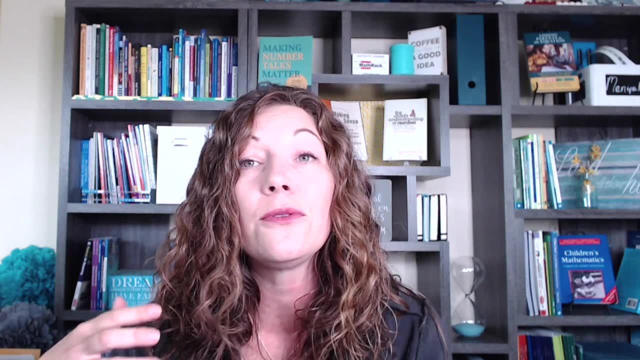 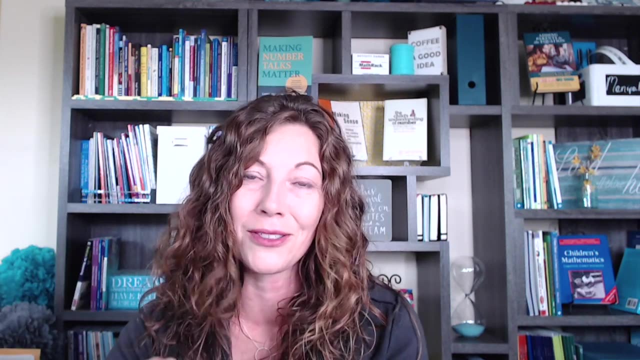 practice. You can't play games if you haven't first yet built some understanding in number sense, Because when you go to play games it becomes frustrating if you can't solve the problems quickly, Because the whole part of games is that you are quick when you're playing those. 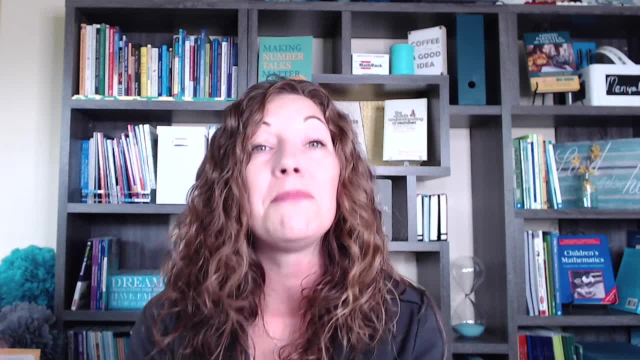 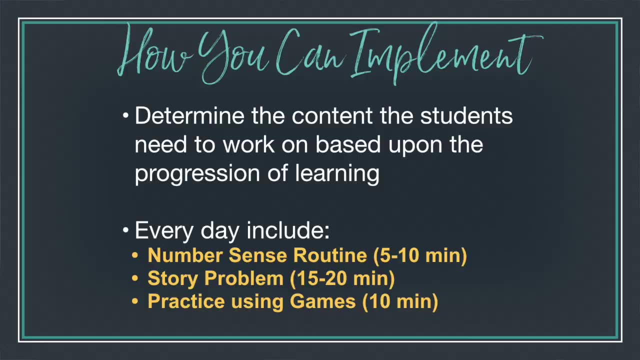 games. So we need to do all of these pieces to help kids build their fluency, And then we just hone that fluency through practice, using these games. Okay, so how do you take these recommendations and how do you practice them? I'm going to show you how to do that in just a 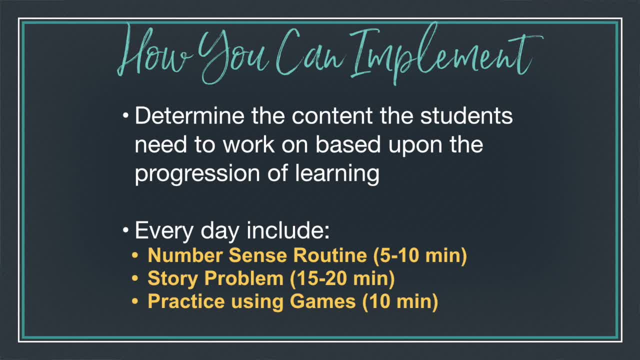 second. So I'm going to show you how to take these recommendations and actually implement them. The first thing- a reminder of my first thing I started this with- is that you need to determine the content your students need to work on, based upon that progression of learning. Then, every day, 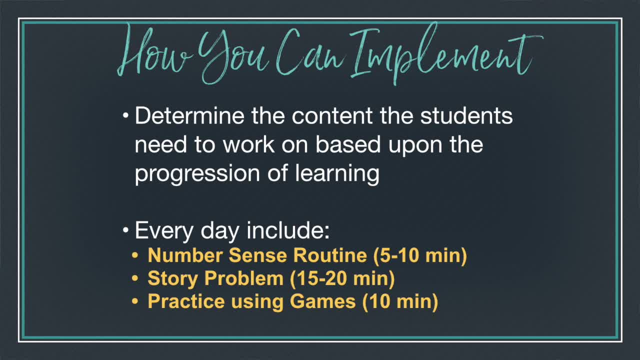 start having some kind of number sense routine. Those routines should not take more than 10 minutes. When you get really good at them, you can do them within five minutes. One of the things I didn't mention- but I will go more in depth with this in future videos- is solving the problem of 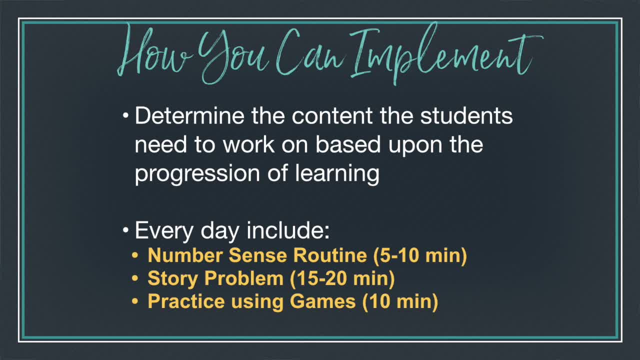 story problems is not just about solving a problem and getting an answer. The big emphasis of story problems is also, then, sharing their thinking and talking about the different ways that kids solved those problems. And then the last piece is to incorporate practice using games. Again, it should. 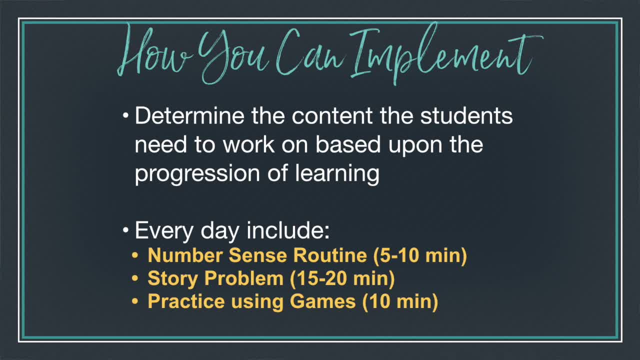 take 10 minutes or less. Once kids start learning evergreen games, all they do is just go pull a game and they can start playing. You don't have to spend time teaching the rules and getting the stuff out. You will have a bunch of pre-made stuff, All right, so I hope that this has given you a little. 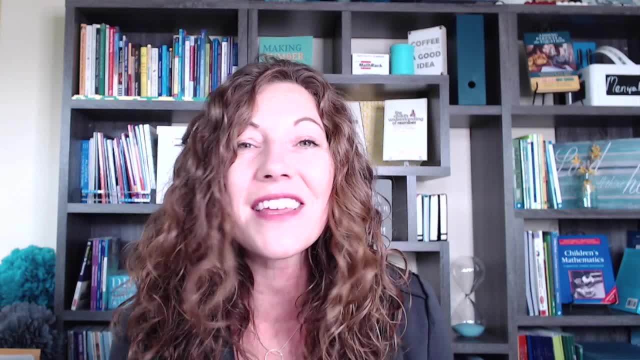 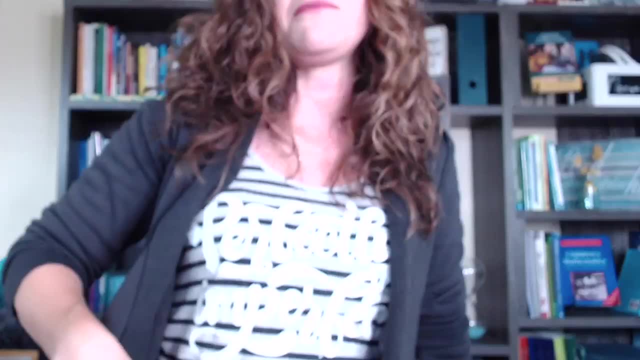 bit of inspiration. Like I said, I hope you take on all of this, But if you don't feel like you can take it all on, just remember I wore my shirt. You probably aren't going to be able to see it. 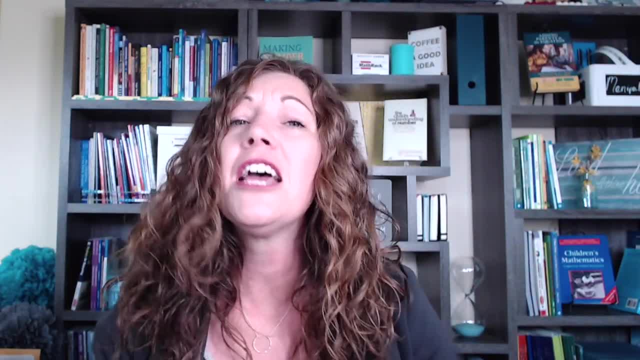 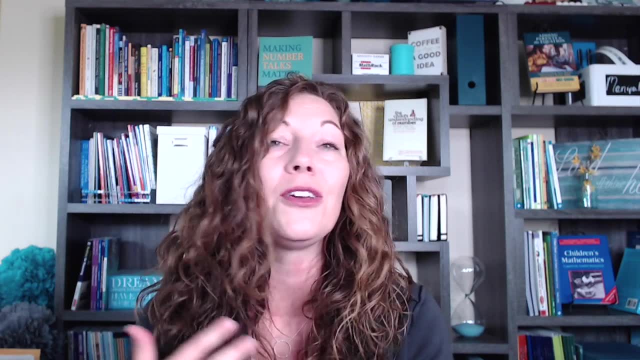 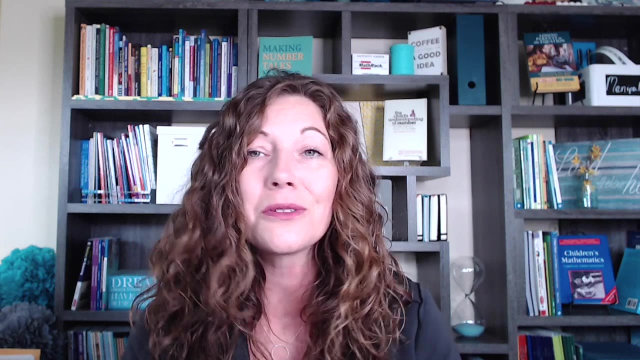 but it's kind of messy here with the stripes and everything, But it's another version of my perfectly imperfect That is. one of my big mottos is that if you are waiting to do this perfectly, it will never happen. Just try something, see how it goes and then implement from there. right, You don't have to do. 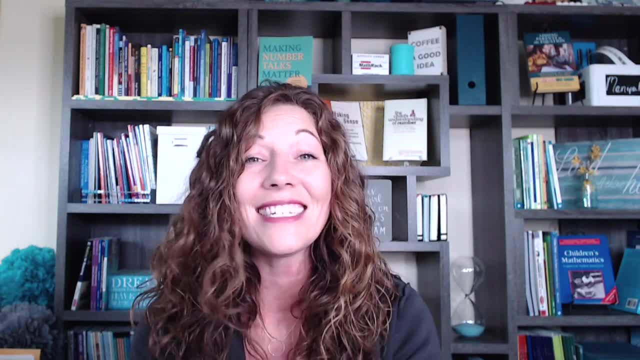 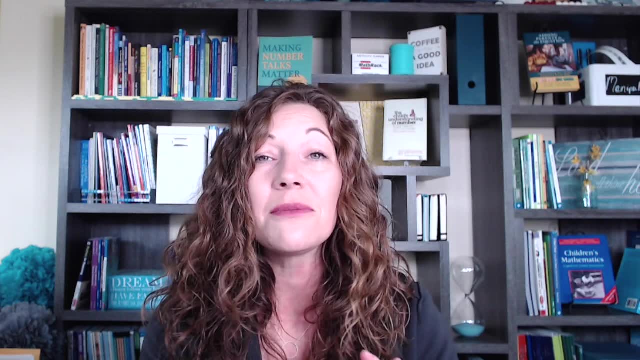 it all at once, So don't forget to download your guide to teaching math without a textbook. It should be right below this video, I outline the reasons why you should move away from your textbook. I give you more detail about the three things that we talked about in this video.